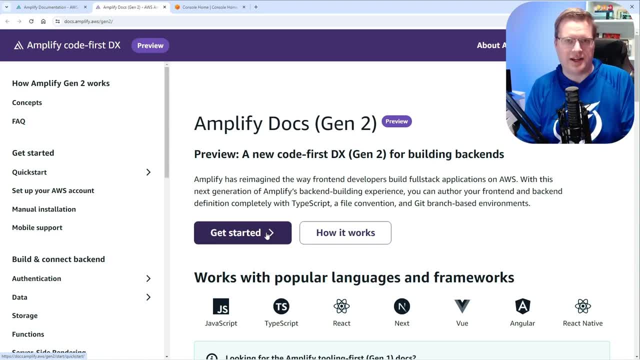 you've been watching this channel for a while, you've probably seen me add in Amplify into some of the Vue projects I've created in the past. So with this Gen2 product it helps you create your back end for your front end websites And it has deep integration so that when you do integrate it, 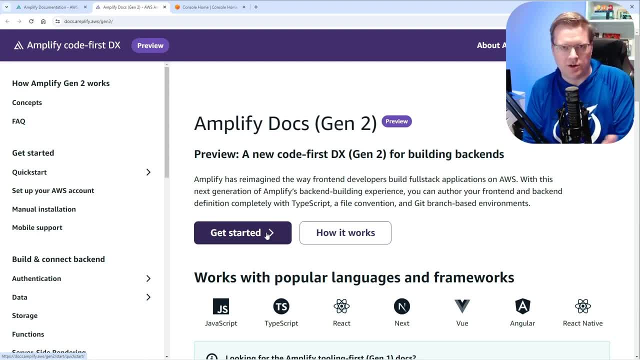 in. you can easily use our libraries to talk to those back end environments that are created, And so, for this first initial release for general, we're going to talk about some of the things that we're going to talk about today. So we're going to 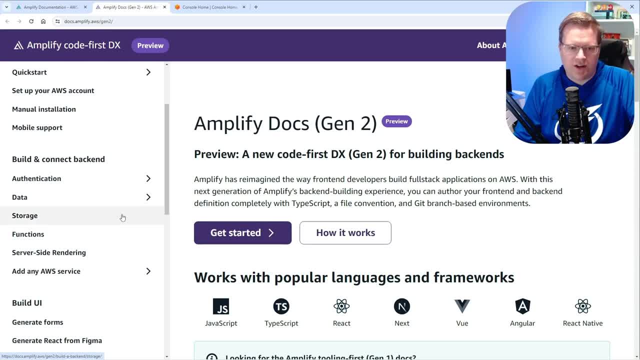 talk about some of the things that we're going to talk about today. So we're going to talk about some of the things that we're going to talk about today. One is availability. We're focusing on four areas. One is authentication. You see your data storage and functions, So authentication. 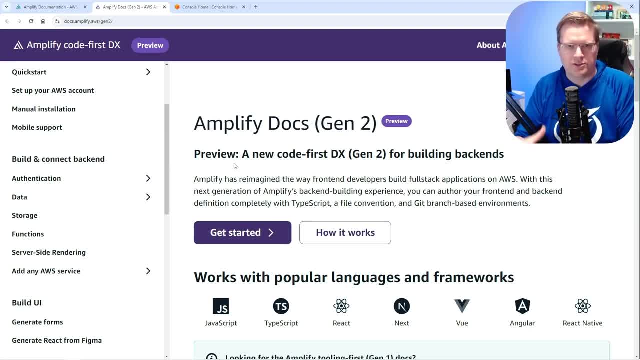 authorization, to make sure only certain people can access your app or certain resources. We also have a data layer that's backed by our managed GraphQL service called AppSync. We have storage, which is backed by S3.. And then we have Lambda functions, So you can create your Lambda functions. 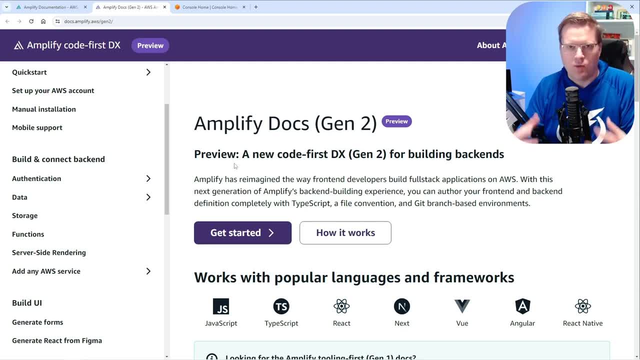 really quickly And we use this infrastructure as code way of doing it. with this code, first developer experience, I think that's going to be a lot of fun. So let's get started, So, let's get started, So, let's get started. So the best way to kind of demonstrate how these work is, we're 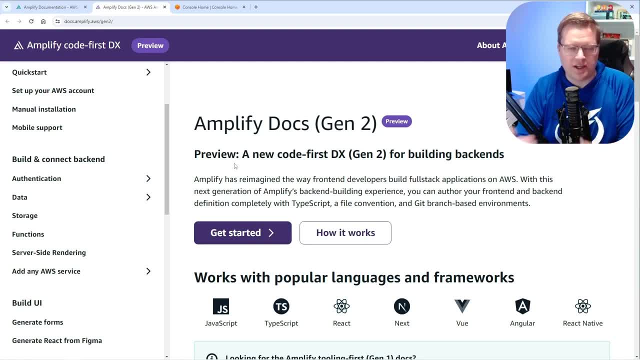 going to create a new app using the console, And then we can take a look at what it generated for us. So to begin, first you'll need to have an AWS account And, by the way, I'll put a link to the. 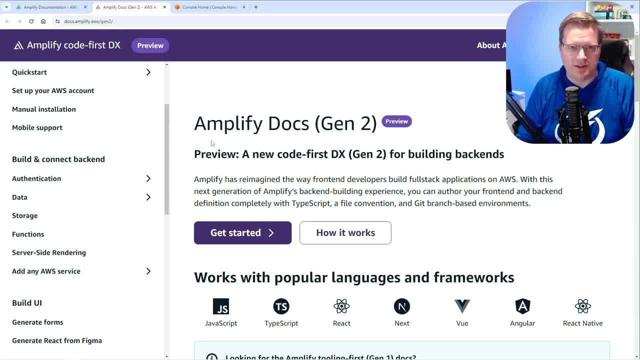 AWS free tier, you get literally 1000s of free hours of time and compute time you can do things with. I would highly recommend checking that out. Other than that, after you create your AWS account, you can log into the console And in the console you just need to search for AWS Amplify. I already 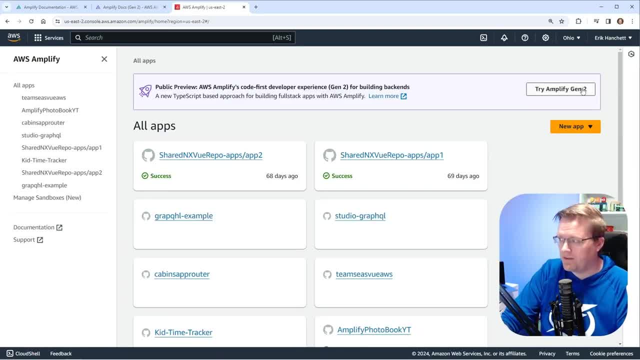 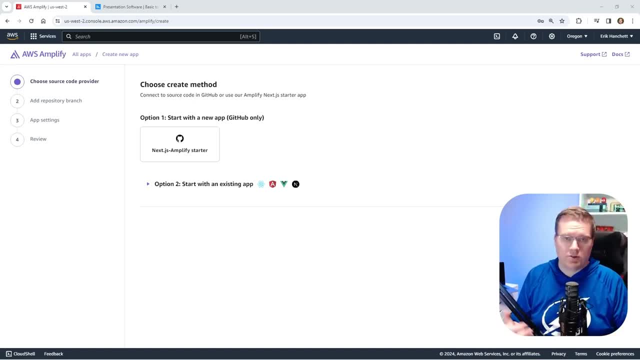 have it here. you just click on it. So right here you can see try Amplify Gen two. So if I click try Amplify Gen two, So on this page it's going to ask us a couple of steps to create our app and 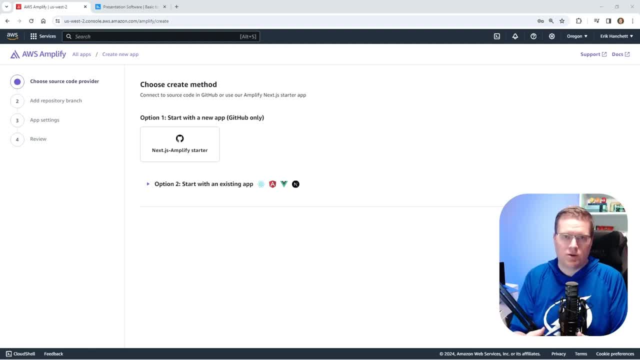 connect it up to our hosting service, which will also deploy our back end. So there's two ways you can do it. you can actually use it with an existing app, which is option two, But today we're going to use option one, which is the Amplify starter app. So what this will do is that there's an 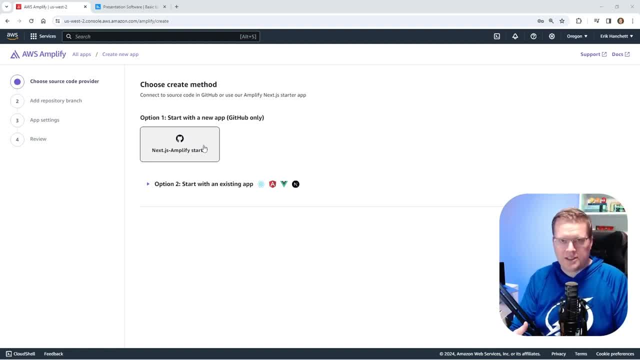 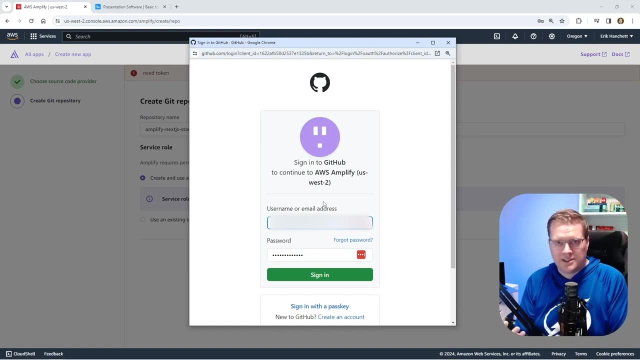 existing GitHub app out there. it'll clone that, I'll fork it into our own GitHub account and then we can use it. So let's take a look. So will you choose NextJS Amplify starter. we'll click next And now it's going to ask us for some permissions, So that way, GitHub has access and we can fork it. 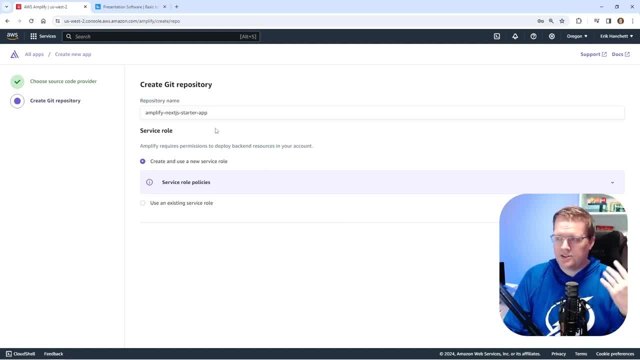 and put it into our account. So I'll go ahead and do that. So now it's on this page, it allows us to add the repository name. So I'm gonna call Amplify NextJS YouTube starter And then I can choose if I. 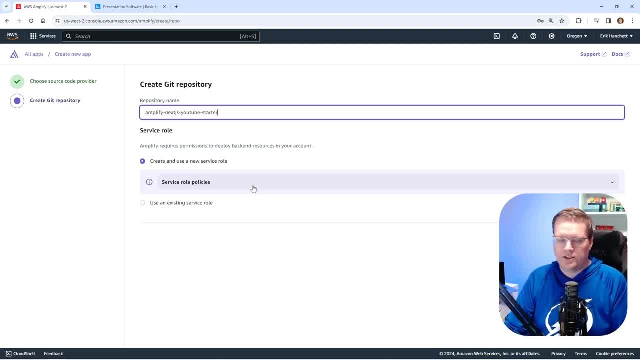 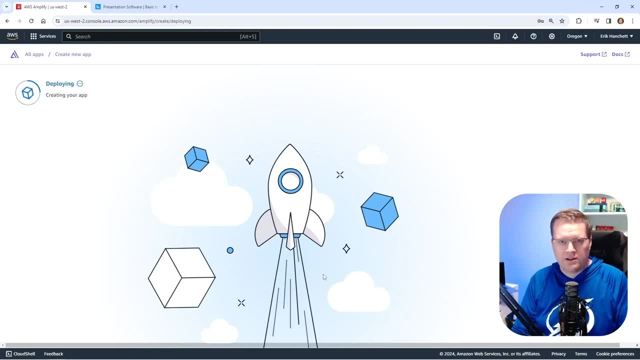 want to create a new starter service role. it's probably best just to create a new service role Now. let's just go ahead and click Save and Deploy. And now what it's doing? it's creating that repository. it's forking down, forking. 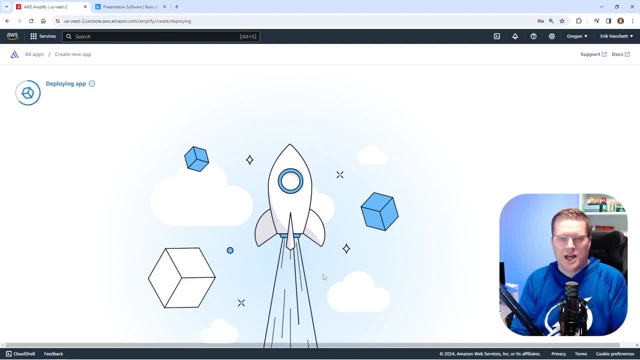 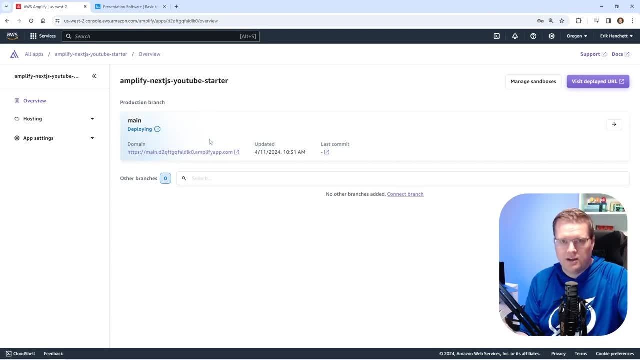 the repository that we have that has some same starter stuff in it, And now we can use it. this will just take a moment. you see, it already brought us to this screen here And what it's doing is it's actually creating the hosting environment. So, app, this app is now hosted on our Amplify. 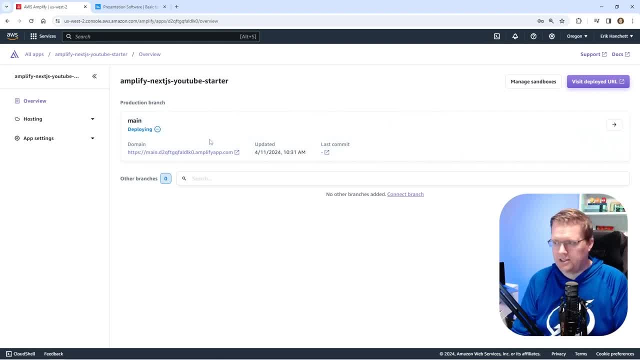 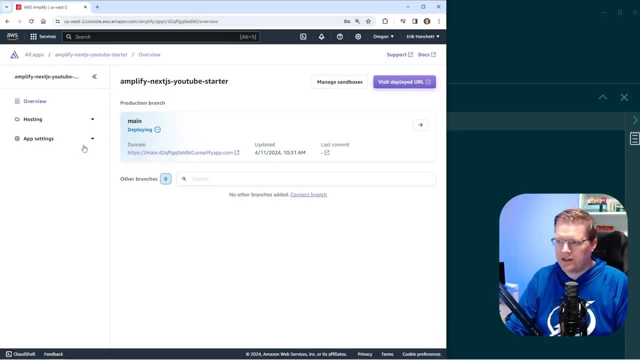 hosting And it's also deploying a back end. Now let's take a look at what the app is that it created for us Now, while it's deploying here, if I click on app settings and then I click on repository settings, it'll connect up to GitHub. 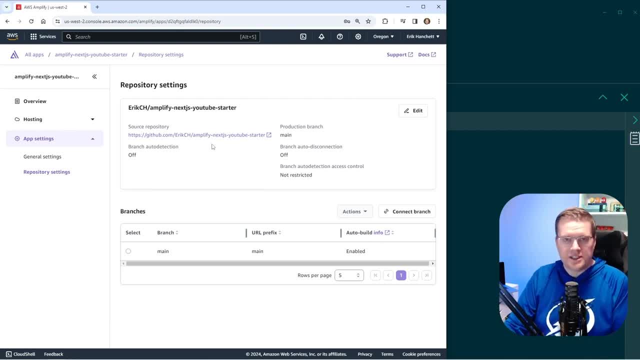 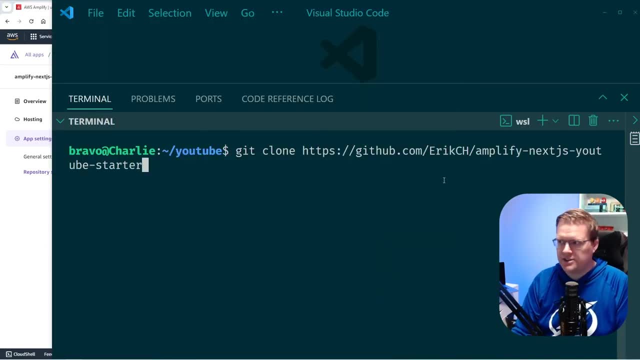 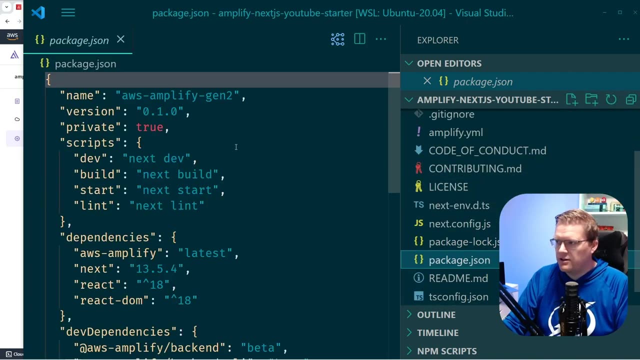 to make sure that we're all connected. And then right here we'll see the source repository. But I'm just going to copy and paste it and I'm just gonna clone it down and take a look at it inside vs code. Okay, so here is the app, But this is the app it created. So next, js app. And if we look here, 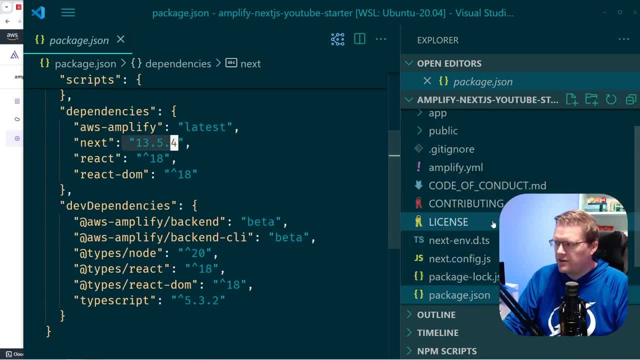 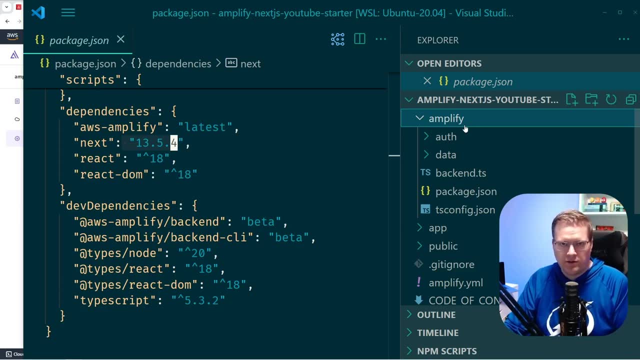 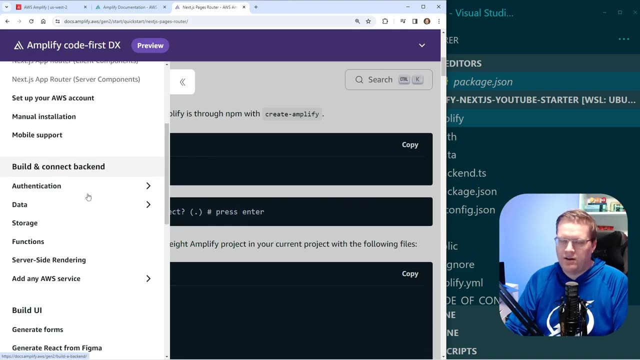 it's using Nextjs 13.5 and the most important thing to realize is, if you use this template, it creates this amplify folder for you, and what this does is, as I mentioned at the beginning of this video, there's really four types of ways you can create. there's four kind of sections in gen 2. 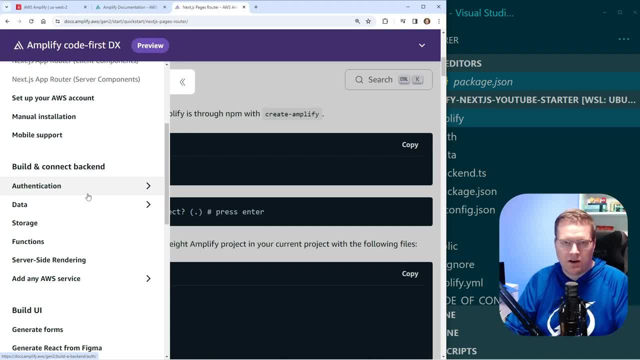 that you can use to create apps, kind of building blocks. there is the authentication layer, which uses Cognito, there's data which is uses or a managed app sync service. there's storage, which uses s3, and there's functions we use as our lambda functions, and so we're creating infrastructure as. 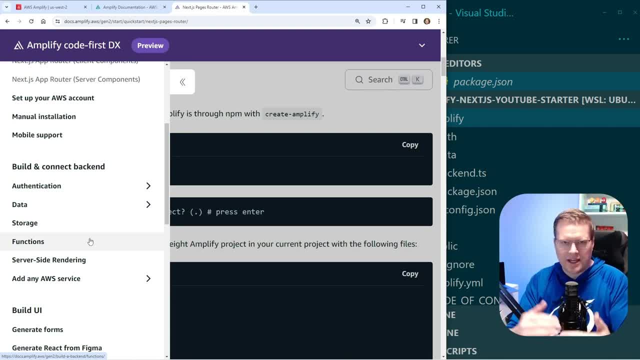 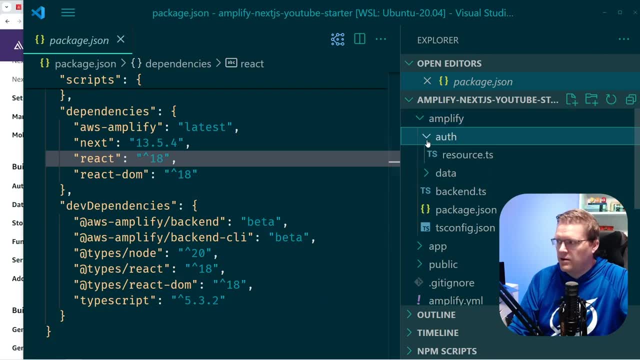 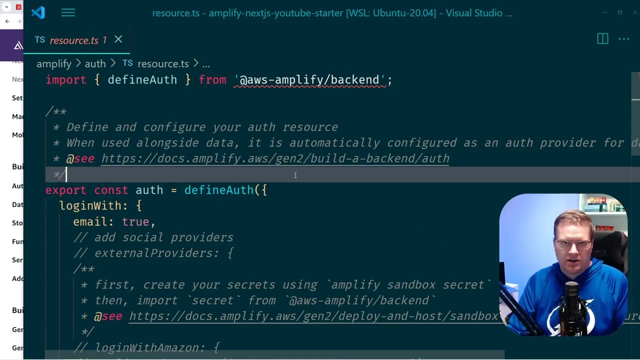 code to create these back-end resources and we have this layer, this gen 2 layer, on it that makes it really straightforward to create these resources. so, out of the box, here it creates a Cognito resource and this is the way you can use this to log in and log out of your app sync service. 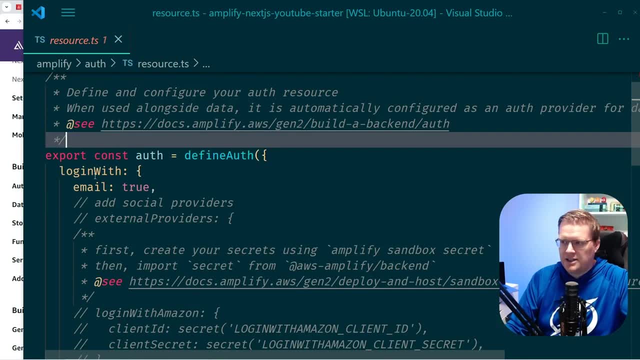 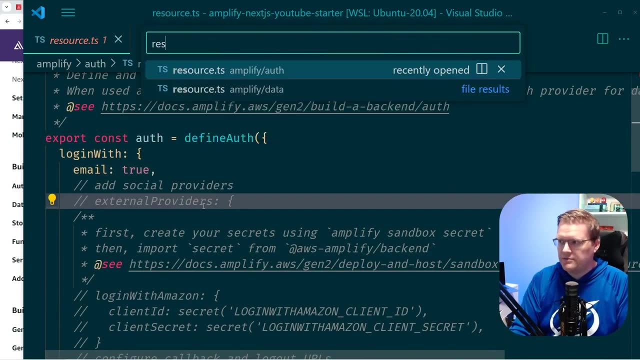 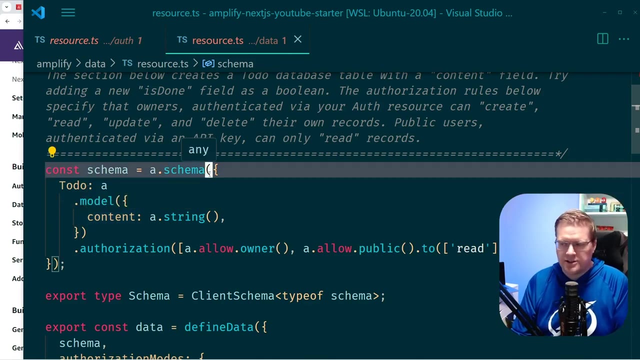 you can do authorization and authentication, and it's set up through email and, of course, we can always change some of these two if we need to. and then it also created a data layer, so it creates this data layer using the managed app sync service, the managed graph QL service, app sync and what 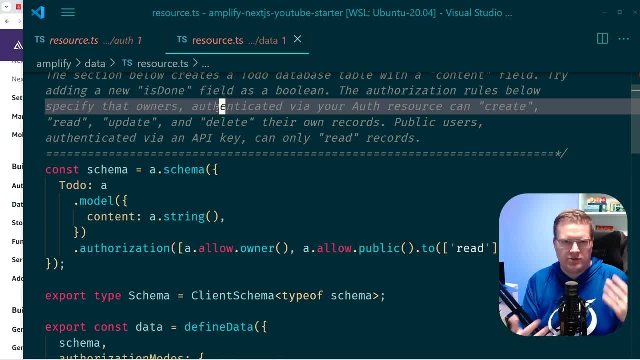 this does it normally with graph QL. you have to create resolvers and resolvers have to talk to different data resources. just by these few lines of code, we'll create all of these resources and we're going to use this to create these resources and we're going to use this to create these resources. 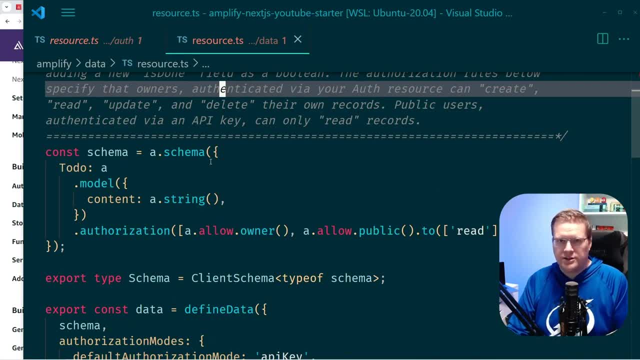 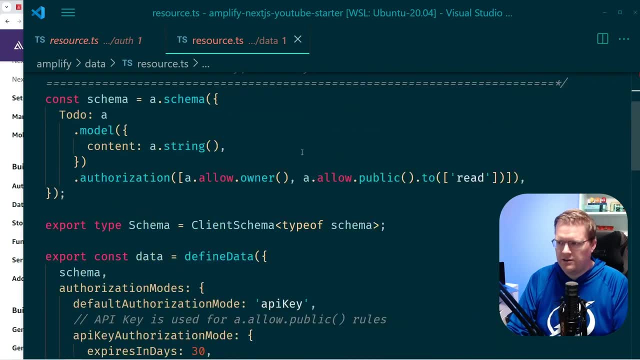 all that for you. so we'll create a dynamo DB database. we'll also create all these resolvers so you can do all the things you normally do- the create, read, update and delete- with this. just this code here. one other thing we'll need to do is when we do npm install, just to make sure everything's. 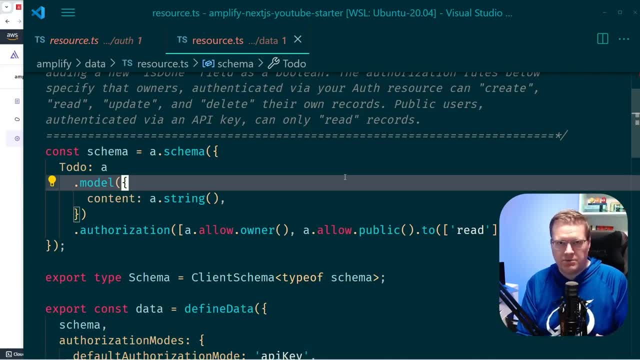 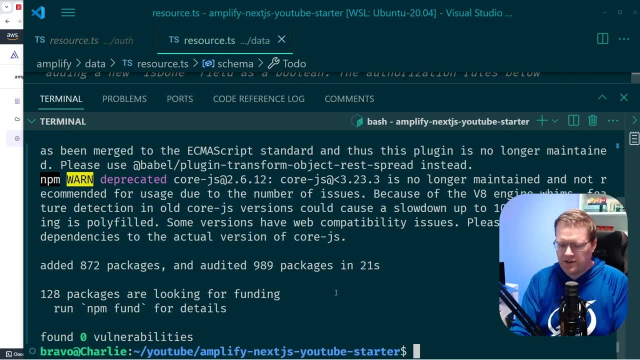 installed. we can make changes to this at any time. we can push it up and it'll update our repository and our hosting at any time. all right, so we have everything started. if I do npm run dev here, we can see here: this is our nextjs app. this. 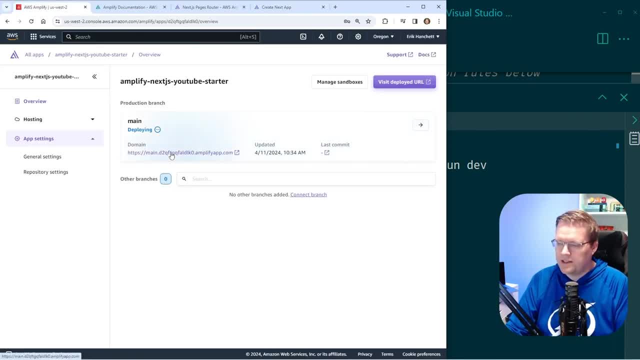 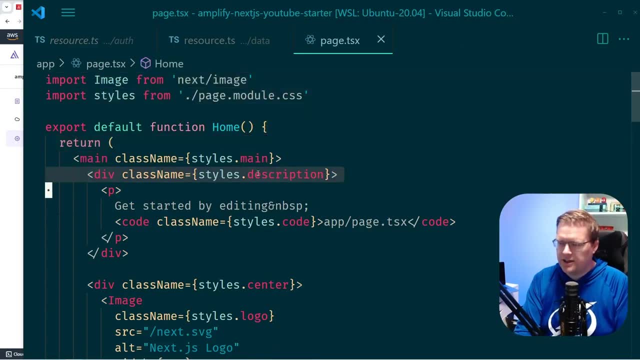 is what it comes out of the box, and if we come back over here once it's deployed, this link right here will go to an app that looks exactly like this. so we can, if we want to start making changes and just do like a hello world if we make the change here, come back over to here. so now we 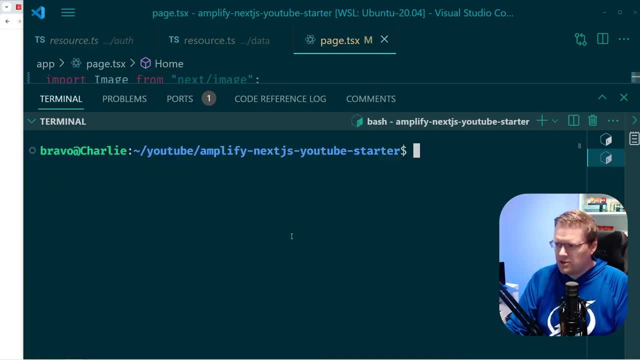 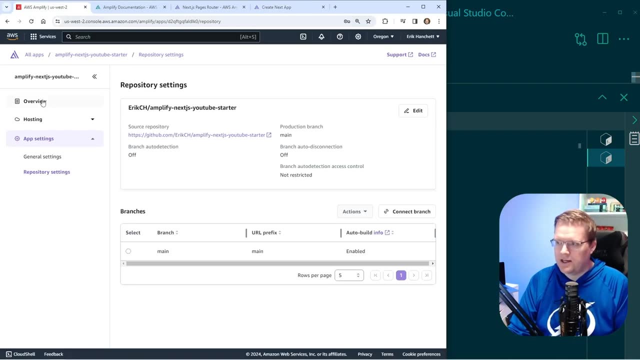 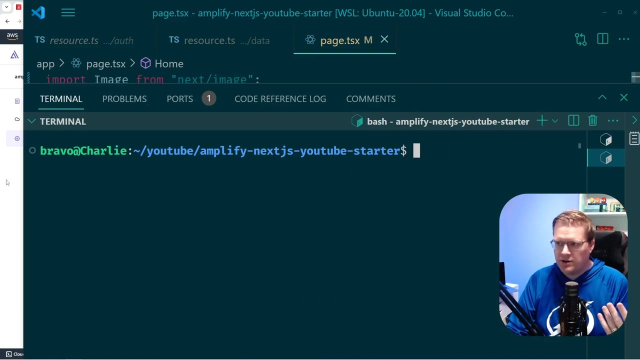 just see hello world as we expect it. if we want to, we can actually create a local environment which is different than this one. so right now, this one is creating a, a production environment for us. so anytime we push up to our repository, it's going to update this URL and you can think of it every. 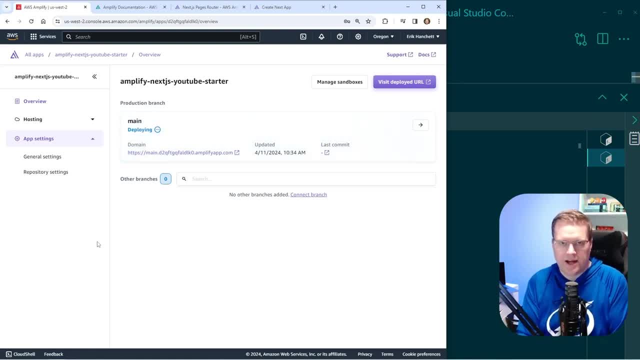 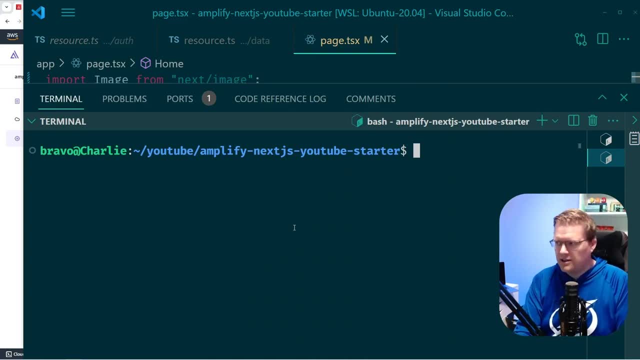 single GitHub branch can be another environment that you have connected to your hosting and your back-end services. but if we want to test locally, there's a command we can do this. there's a command we can use to do this. so we can do mpx, amplify sandbox, and obviously you only have your AWS. 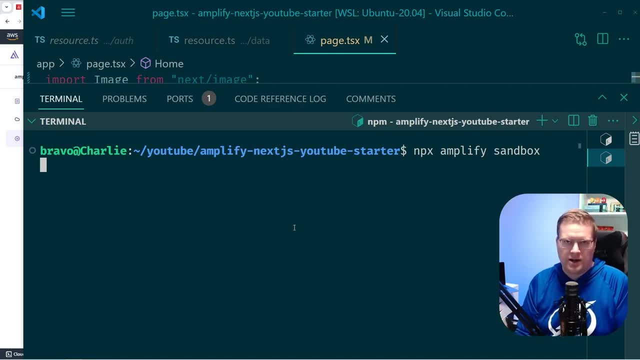 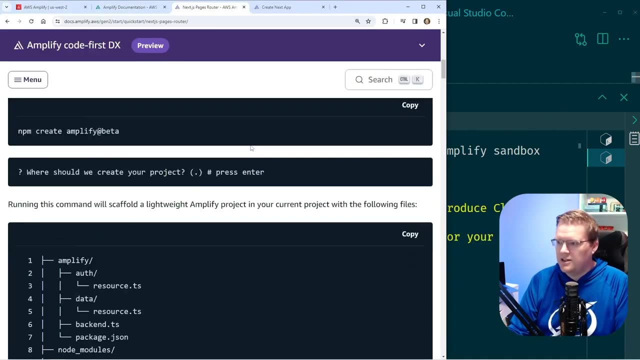 account. if you don't have it set up, this will give you an error and it'll give you some instructions locally. if you don't know how to do that, you can always look at the documentation it's in here. configure your AWS account to use amplify. so there's a few few steps that you'll have to do. 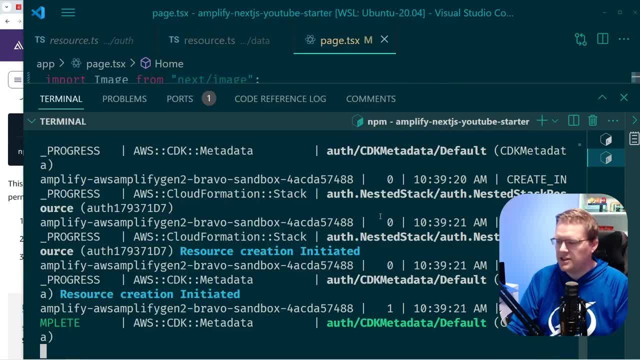 that, including running this npm, amplify, configure, but I'll assume that you did that. now, if I'm running sandbox here, it's going to actually create an ephemeral environment that I can use to test our app locally. so the production environment is completely separate. this will be our local. 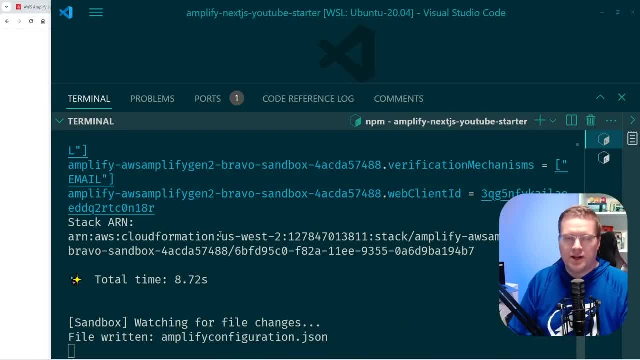 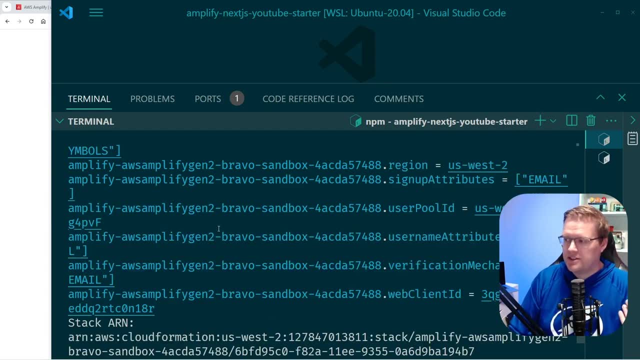 environment, so we'll just give it a second for this to start. all right, so our sandbox is done and it went ahead and created an ephemeral environment that we can now use to test with and you can see, it outputted a bunch of data for us and it created 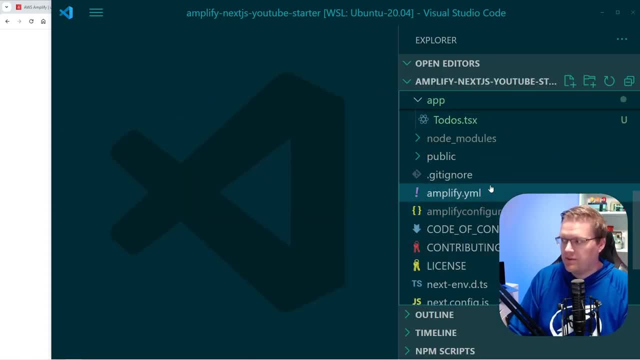 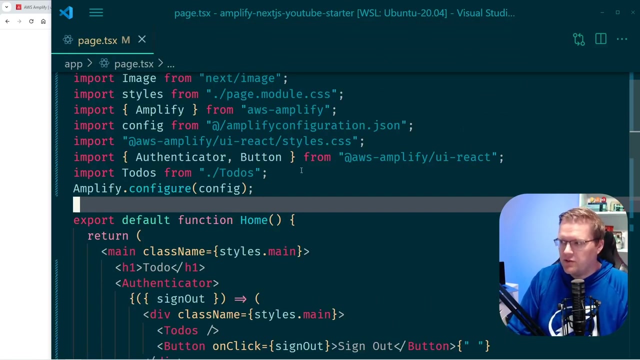 a new folder, a new file actually called amplify configurationjson, in the root folder of our app, and we can use this to help test locally. so to do this, I went ahead and added in some code. for the sake of the length of this video, show you what I did. so we can test this out. if I go into the pagetsx file, I added in some, a few. 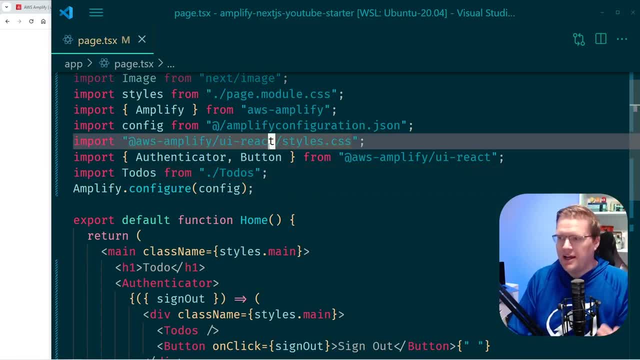 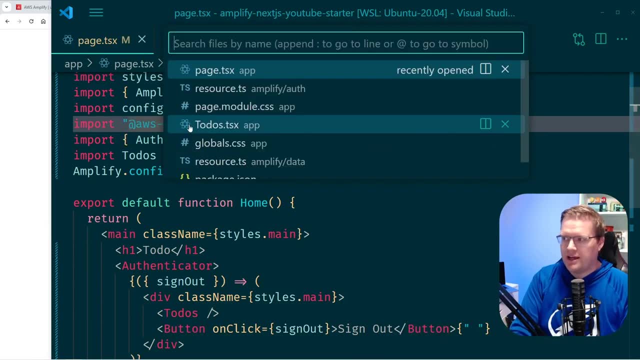 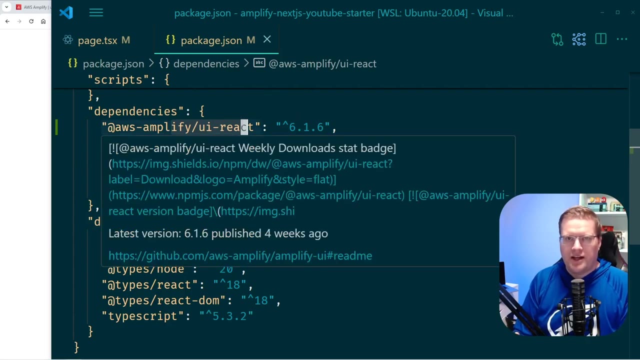 things in here. so, as we look at this file- and I'll put a link to this in the description if you want to look more closely- I installed a new library called amplify uireact. so this library- right here it's a component library that has some boilerplate code that you can add to add in extra additional. 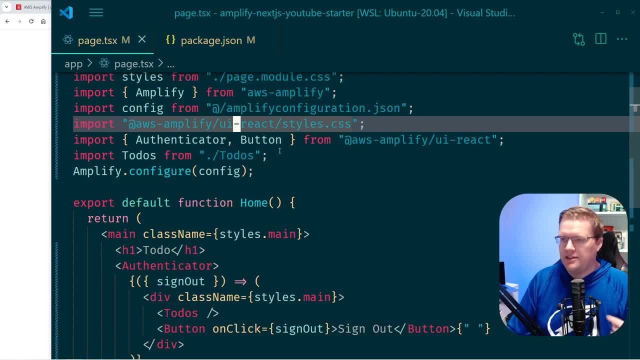 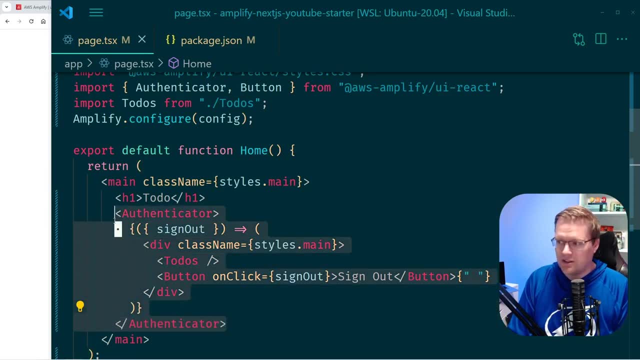 AWS Services, and one of them is the authenticator, and it also includes a whole component library, so I'll show you this. so this authenticator allows us, with just these I don't know five, six lines of code, to add in a login system to our app and it will automatically connect up. 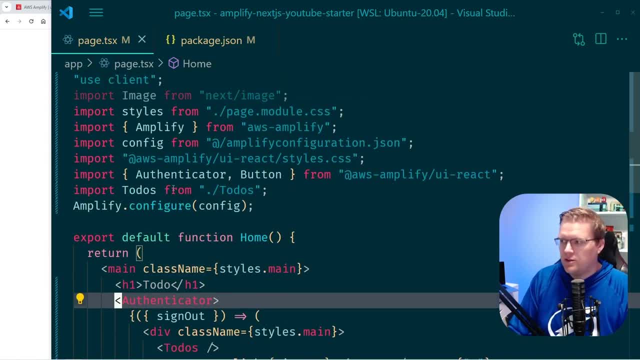 to our resources that we've already created. I also installed this configure. I added this amplifyconfigure and what this does is it takes this file. I'm importing in the from the Amplify configuration JSON file. I'm importing an Amplify and configuring it, so everything talks together. 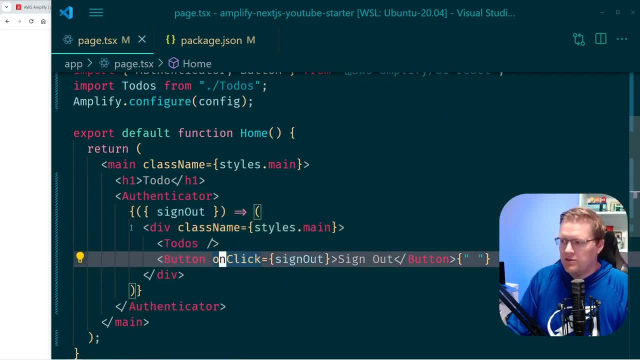 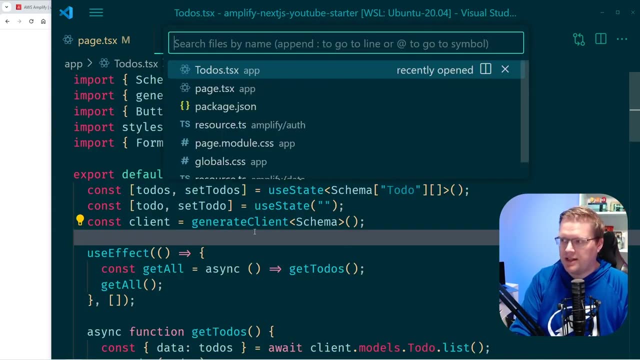 And so for the authenticator I'm saying, once you log in, you'll display this data, including this new to-dos. So if we look at to-dos, by default there's this if you look in the packagejson: 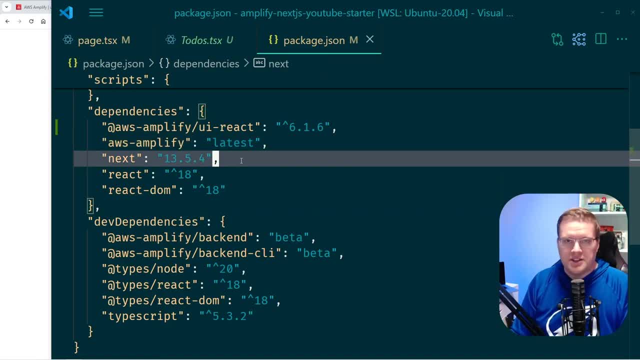 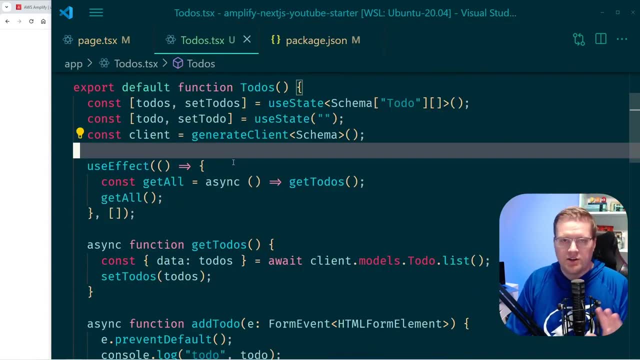 it installed this AWS Amplify latest. So this is the library that will allow us to connect to AWS services If we go to our to-dos. I just created a very straightforward way to add and display to-dos. I didn't add any way to delete them. 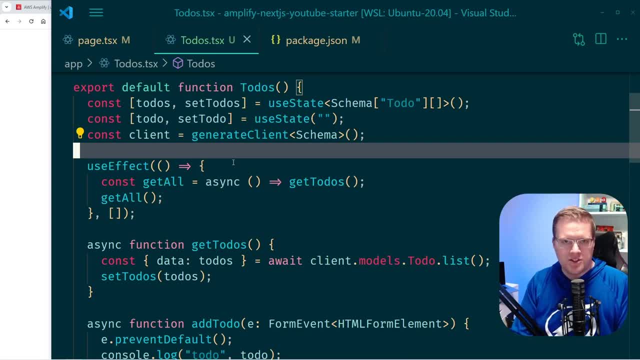 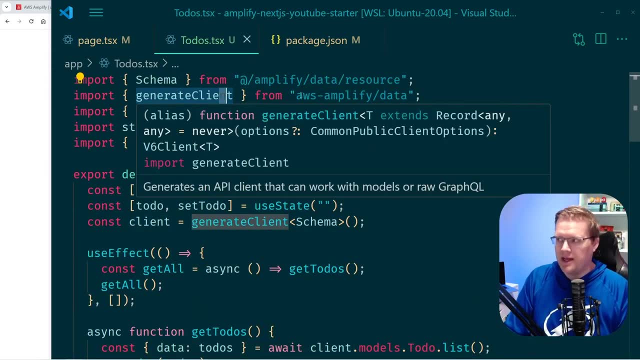 but certainly, if you're following along and watching this, see if you can pull down this repository and add a delete function. I'm using this client And one thing nice about this is I'm using this generate client from the AWS Amplify library. 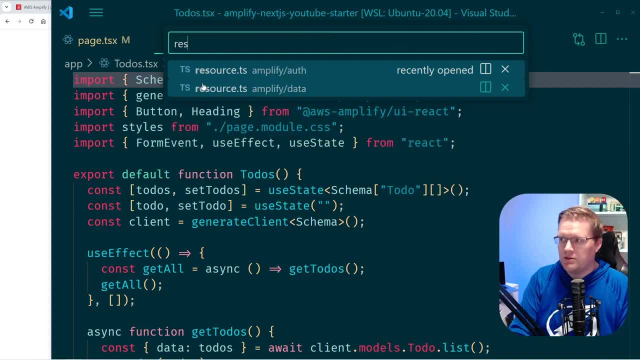 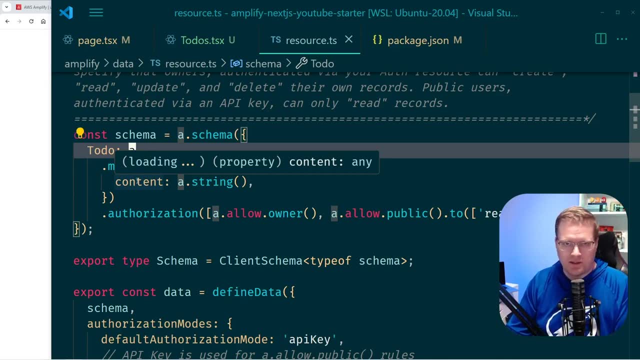 and I'm also passing in the schema. So, if you remember, earlier I showed you that the schema to add this to-dos was defaulted in here. I didn't change anything, I just left it as default. but we could certainly make it. 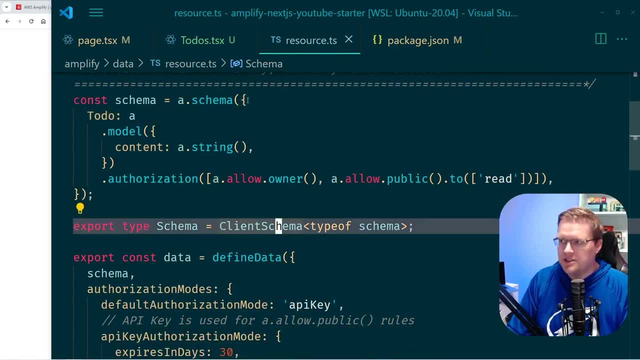 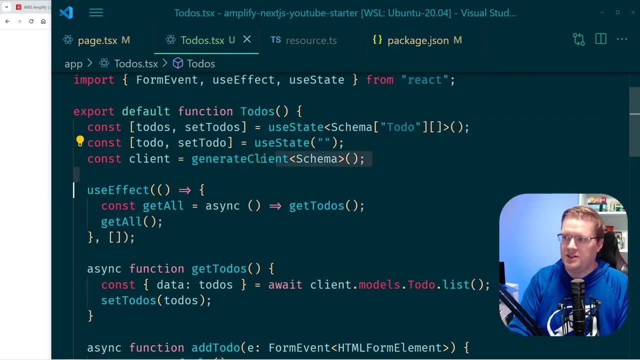 to whatever we want it to be, But it exports this schema type, And so now I can import that schema type into my generate client and now I get full type safety. So, for example, if I type in clientdot, now I can see everything I want. 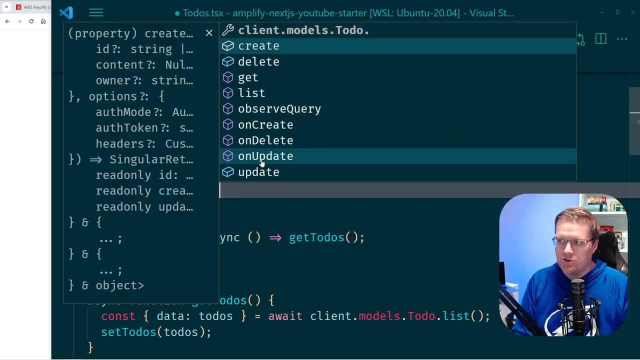 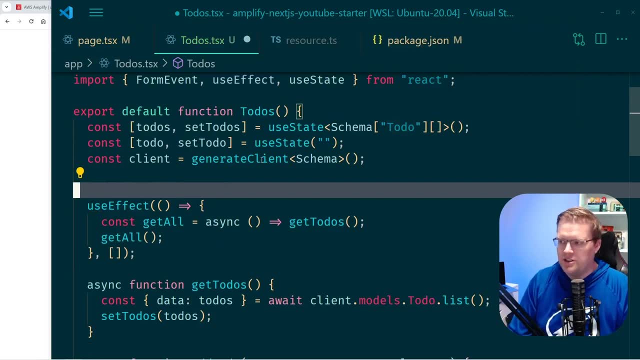 I can do models to-do, and here's where I can do create, delete, get list. I can do observes, queries, all these other things, and it's all typed for me, which is really straightforward and nice. So if we look at get to-dos, 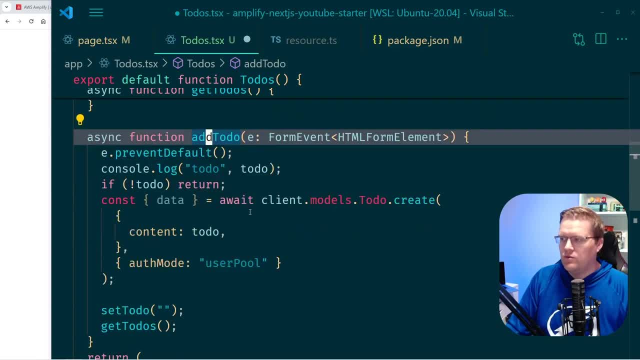 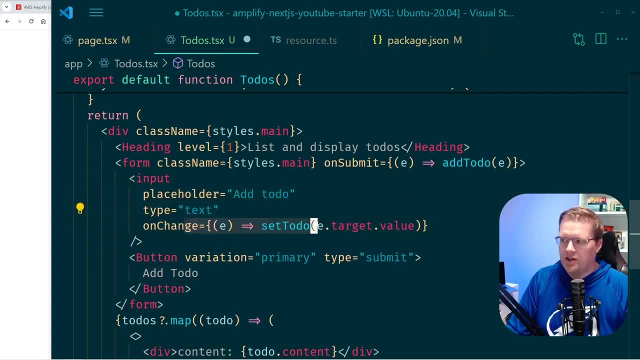 I'm doing a list and then I added an add to-do which automatically adds this content. So I have this input right here. with add to-do, I have an on change handle with a use date to set it, and then I have a submit button. 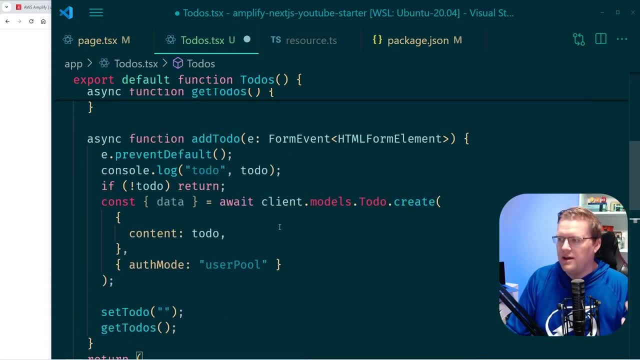 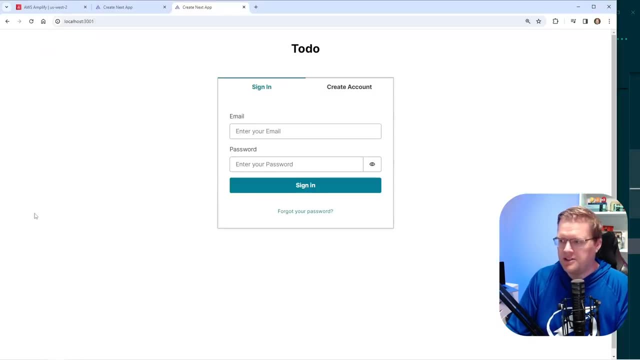 So anytime you hit enter, it submits the add to-do and it creates this new to-do and then it lists it. So let's take a look at and see how this works. First, this is the authenticator. It came out of the box. 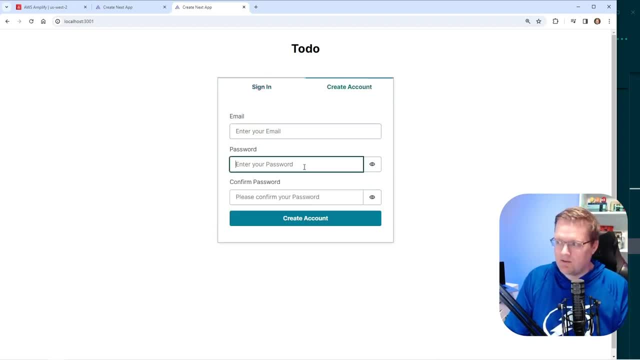 I didn't have to do anything here. What I can do is I can create a new account right in here, create a new account and then sign in. I went ahead and did that off camera, So I'm gonna go ahead and just sign in real quickly. 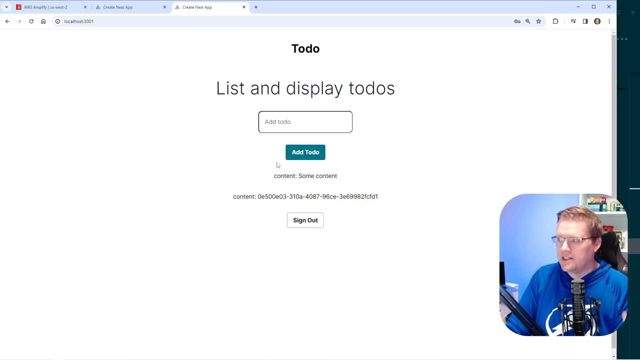 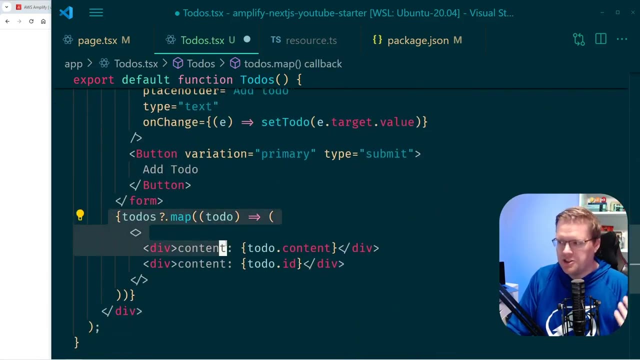 and enter my data in. All right. so it just signed in and here it is. I went ahead and added one piece of content in here. You could see right here I'm just doing a map just to list the content and ID. 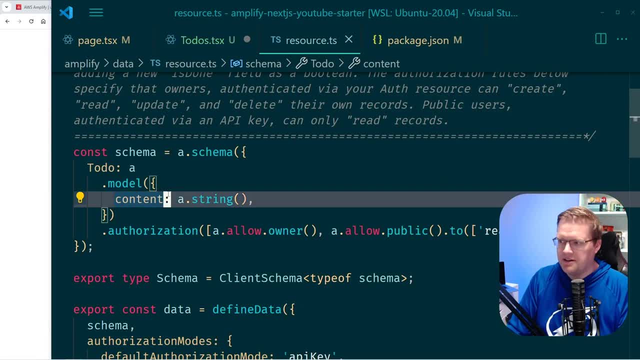 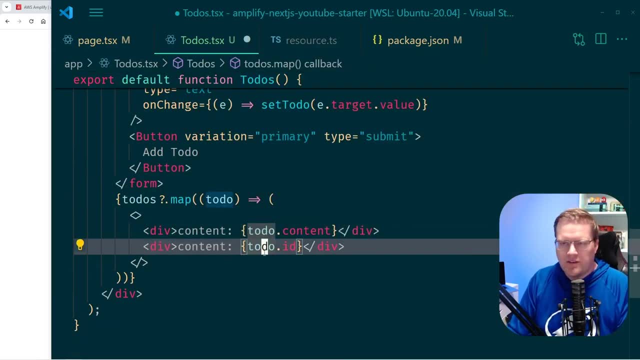 If you look here, all I have is this content. So that's all I have. It's a very, very simple model, And then you also have an ID that it just automatically creates for you. So if I come back here and I add: 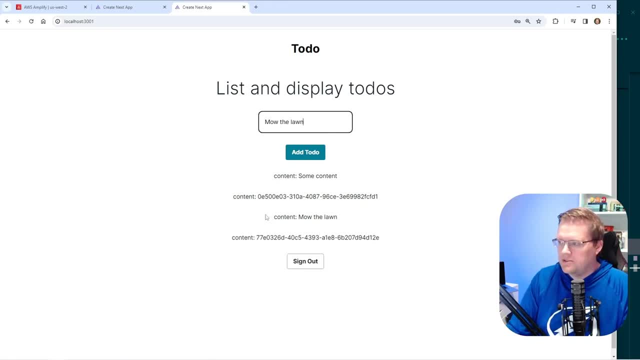 let's say a second to-do, like. let's say, mow the lawn. here it is, mow the lawn is at the bottom, So I can also at any time sign out. Now you're thinking like this is an ephemeral environment. 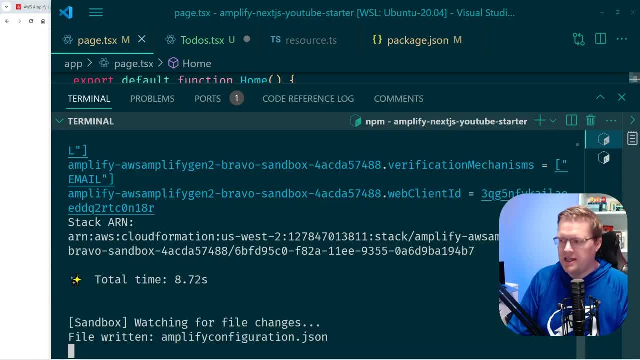 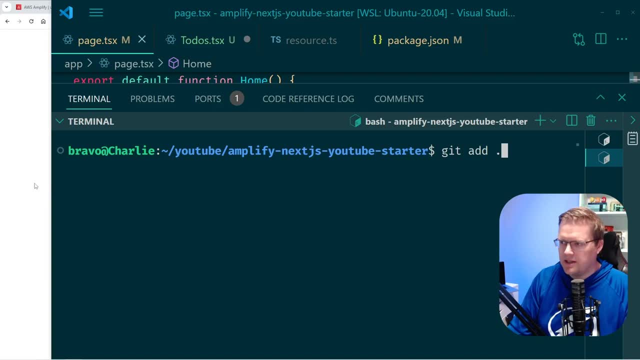 This isn't my production environment. Let's say, I wanted to have this be as production. Well, all I need to do is I need to add here: So if I go back to my console, so real quick, we haven't pushed anything. 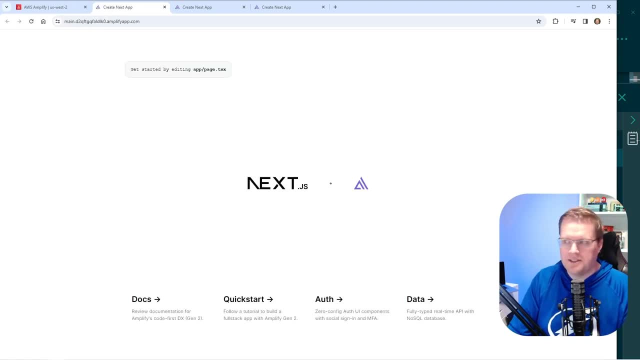 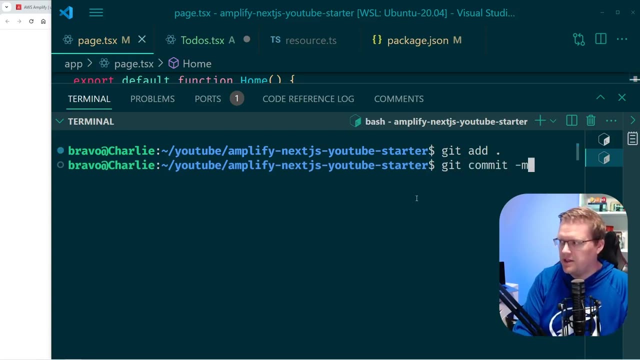 So if we click on this, it still shows the old template. If we want to push this production or whatever branch we have set up, I'm just going to add it, I'm going to commit it First commit, And then I'm going to push it back to my repository. 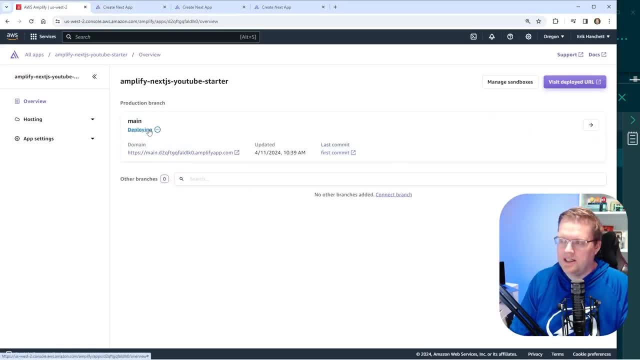 And you'll see right away if I come back here and we could say: see a second. now it's deploying again, So it's checking to see if any changes to our Amplify backend And also chain making any updates to our front end. 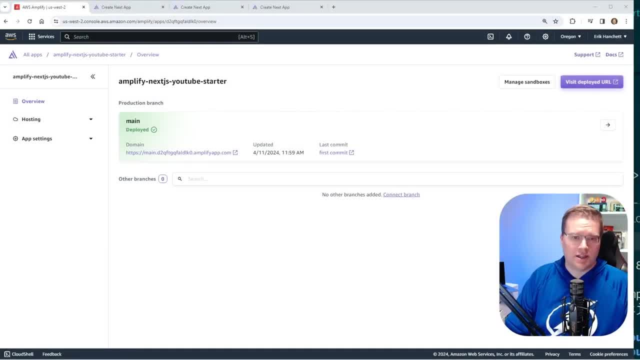 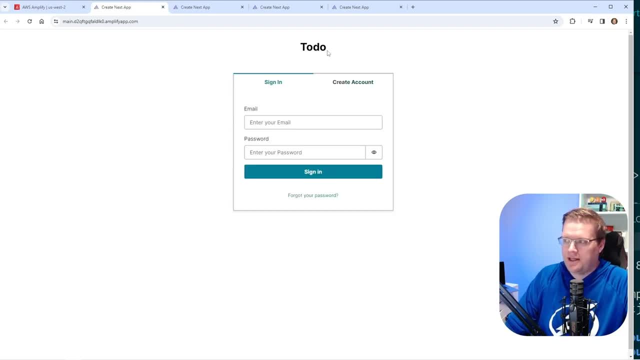 So let's give this a second and see if it updated in production. Okay, it says the resource is deployed now And if I click here, and this is my production account, if I click here, oh great, I can log in. 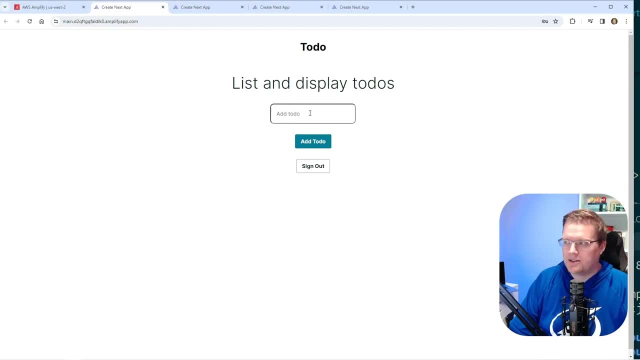 Let's, I'll log in real quickly. I'll create a new account. All right, so I'm logged in And, by the way, this is completely new information. This isn't the ephemeral environment, So I don't see those to do's I created on that environment. 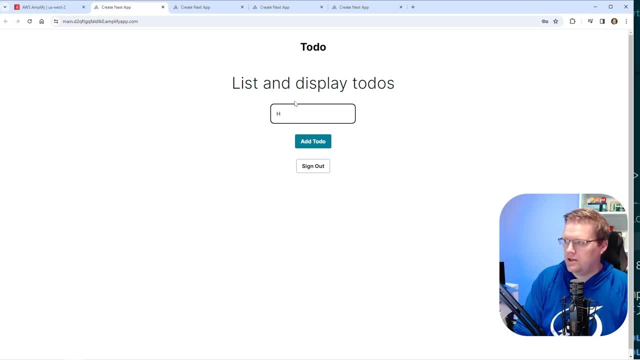 This is brand new And if I do mow the lawn and I click on that and enter- great, So it's now connected to my new production app- Awesome. Let me know what you guys think of Gen2.. Leave a comment below.